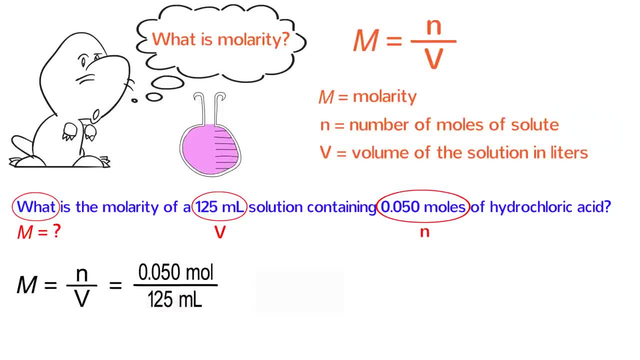 volume. You may be tempted to write 125 mL in the denominator, but that would be incorrect because v should be the volume in liters, not mL. In order to convert 125 mL to liters, you can multiply it by conversion factor fraction. Because 1 liter equals 1000 mL, we put 1000. 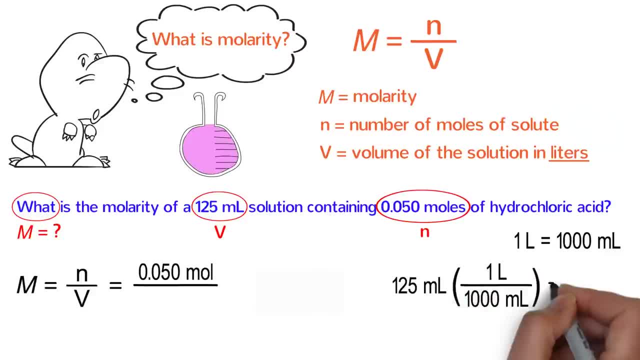 mL on the bottom and 1 liter on the top, The volume works out to be 0.125 liters. However, because we are dealing with metric prefixes, we could have done the conversion simply by moving the decimal point according to the prefix For milli, just move the decimal point. 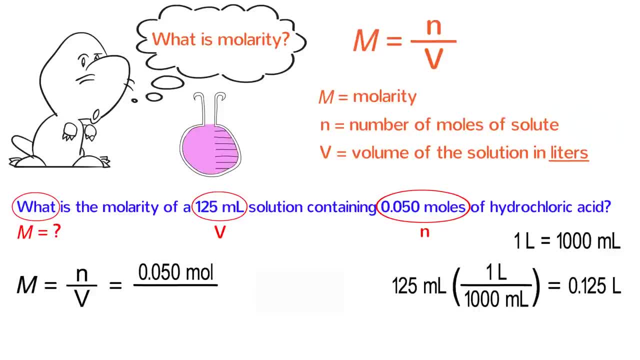 three spots to the left. Back to the original problem. v equals 0.125 liters, so put that in the denominator, Do the division and the answer works out to be 0.40 moles per liter. In general, the units of molarity are moles per liter. 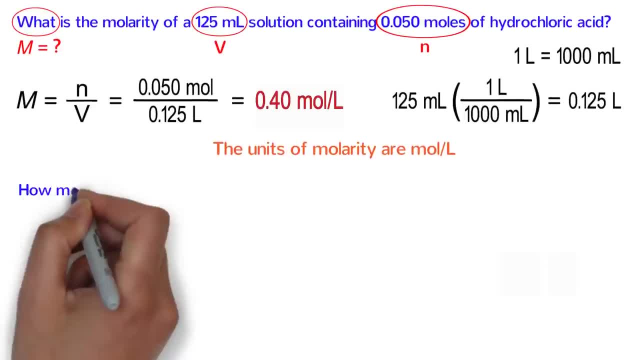 Let's try another problem where we are solving for something different: How many moles of sodium hydroxide are in 38 mL of 0.5 moles per liter sodium hydroxide? The problem is asking us to calculate moles and it tells us that the volume is 38 mL. 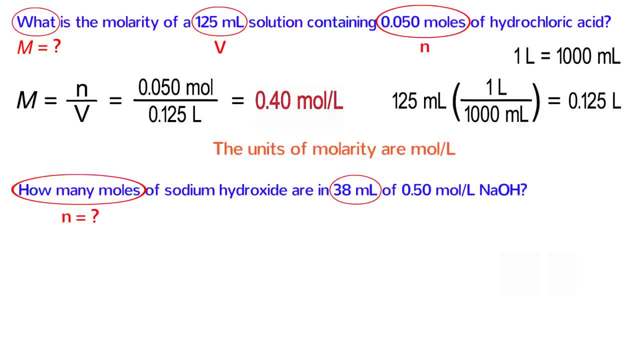 However, for molarity, we will need to convert that to liters, which we can do simply by moving the decimal point three places to the left. 0.50 moles per liter is the molarity. Next, write down the appropriate equation: m equals n over v, Because we are solving. 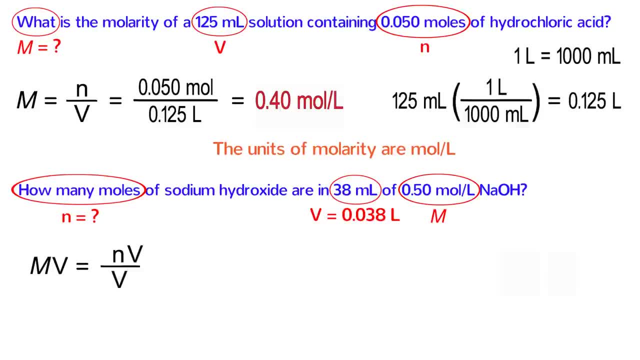 for n. we multiply both sides of the equation by v. On the right side, v over v cancels out, leaving n all. but We can rewrite the equation as: n equals m times v. Plug in the values for m and v, remembering. 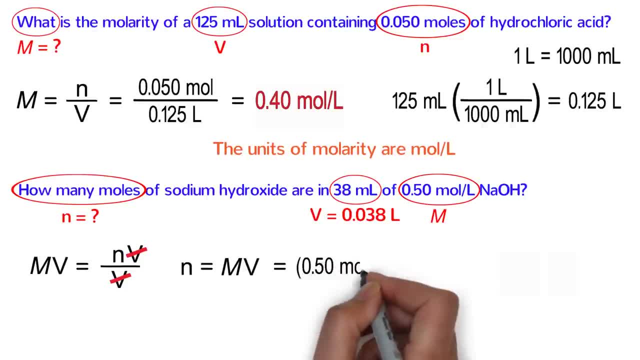 that v has to be in liters. 0.5 moles per liter times 0.038 liters equals 0.019.. As for the units, liters on the top and bottom cancel and the answer has the units of moles. 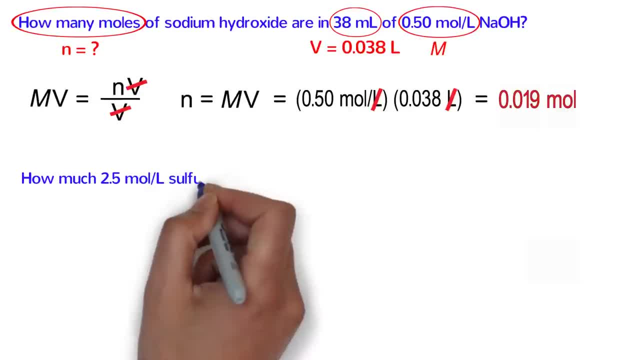 Let's try another one. How much 2.5 mole per liter sulfuric acid should you use if you need 0.12 moles of sulfuric acid? This problem simply asks us how much sulfuric acid, which is a little vague. but think about what you would do in a lab. How would you measure out? 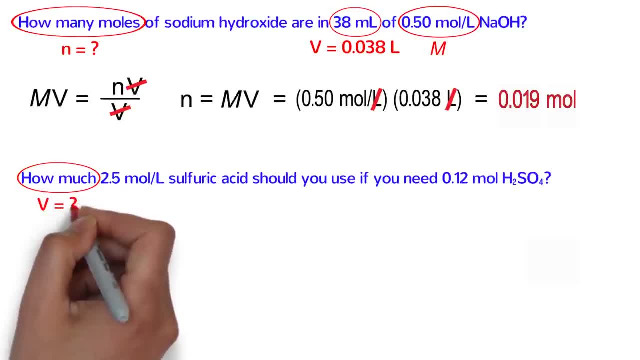 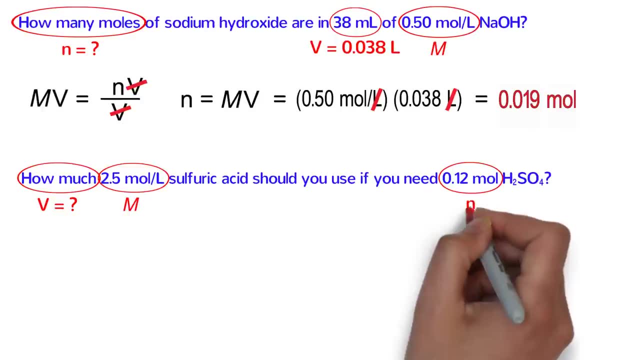 a solution of sulfuric acid By its volume, of course. So the problem is asking us to solve for volume: 2.5 moles per liter is the molarity and 0.12 moles is n. Next write down the appropriate equation. We use n equals m times v, because it is closer. 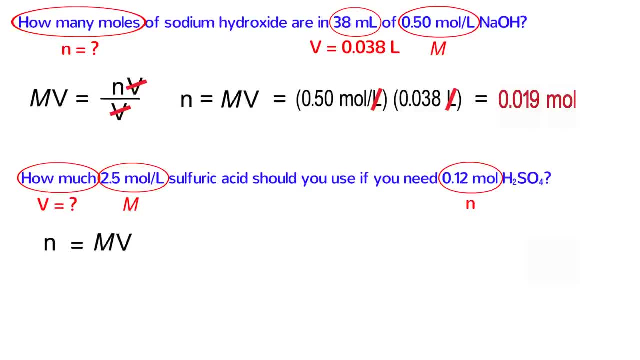 to 0.2.. SUB. just as n equals m and v comes from the past dear us. In order to get v, divide both sides of the equation by m. On the right side, m over m cancels out, leaving v all by itself. We can rewrite the equation as: v equals n. 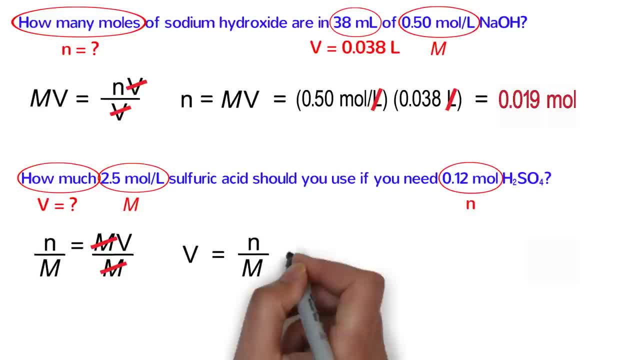 over m. Finally, plug in the values for n and m: 0.12 moles divided by 2.5 moles per liter equals 0.048.. As for the units moles on the top and bottom, cancel, leaving us with. liters as the units. If we're going to get v all by itself, we should only write a simple number in process, Just add in 1. Run the desp 따or one rate knockdabra. So right now you have 0.02 moles And结ğim. 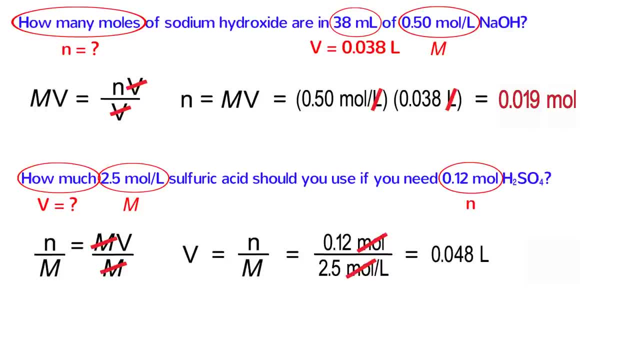 703 moles per liter equals 0.088 liters per liter A from all of the chorus to revenue equals. Because the number is less than 1, we convert it into milliliters by moving the decimal point 3 places to the right, giving us the final answer of 48 milliliters. 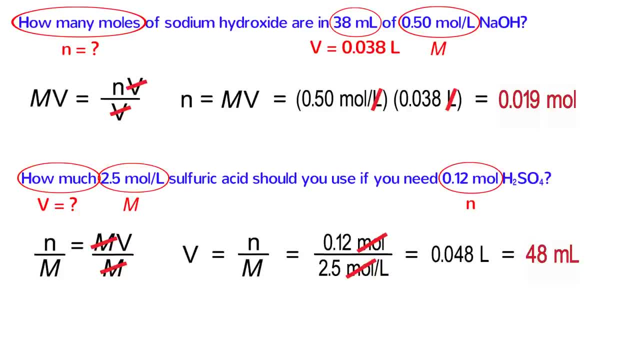 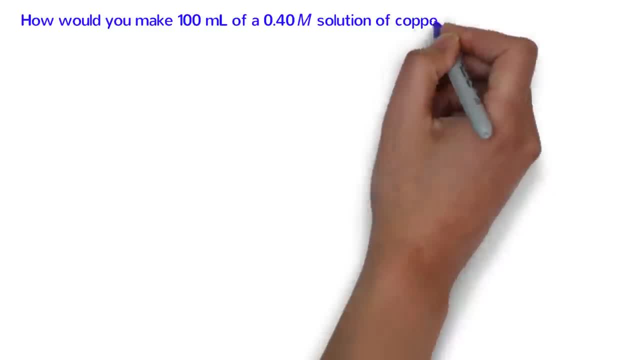 Now for our final problem. Let's talk about how you would actually make a solution of a given molarity. How would you make 100 milliliters of a 0.4 molar solution of copper sulfate? In this question we notice something different: 0.40m. 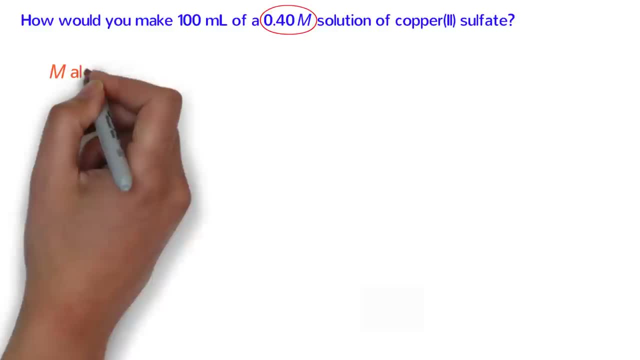 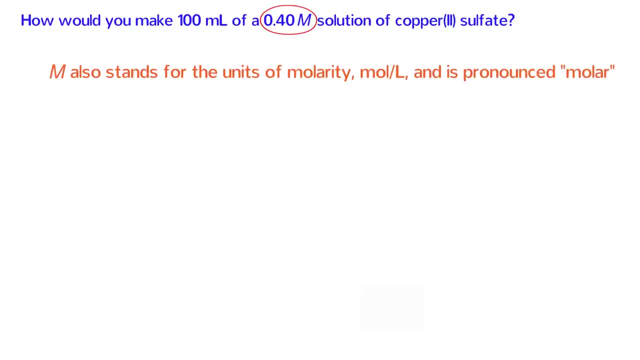 That italicized M not only stands for molarity, but it also stands for the units of molarity- moles per liter- and is pronounced molar. So a 0.4 molar solution is the same as 0.4 moles per liter. 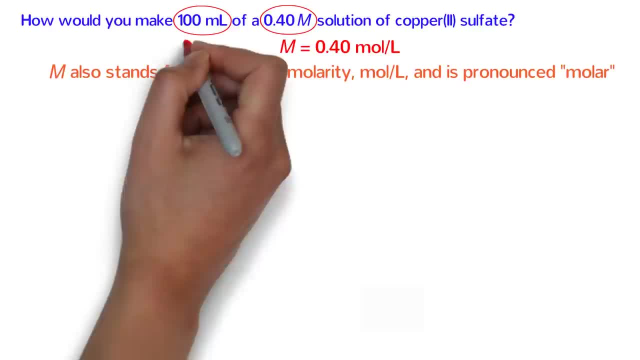 The volume of the solution that we need to make is 100 milliliters, which is the same as 0.1 liters. This problem is more complex than the previous ones, but let's go ahead and solve it, like the previous problems. first. 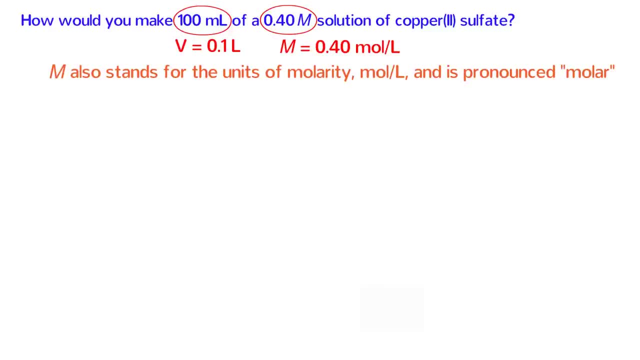 If we know V and M, then we can calculate M. M equals N over V. rearranges to N equals MV. Substituting in for M and V gives us 0.4 moles per liter times 0.1 liters Liters on the top and bottom cancel and the answer is 0.04 moles. 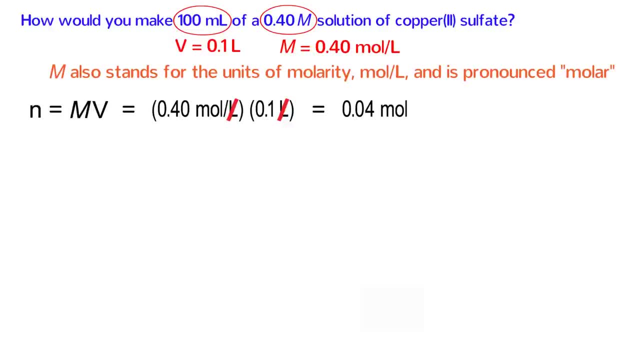 But if we are going to make this in the lab, we need to know how much copper sulfate to weigh out. So we are going to convert the moles into grams. In order to do that, we need the molar mass, which is our conversion factor. 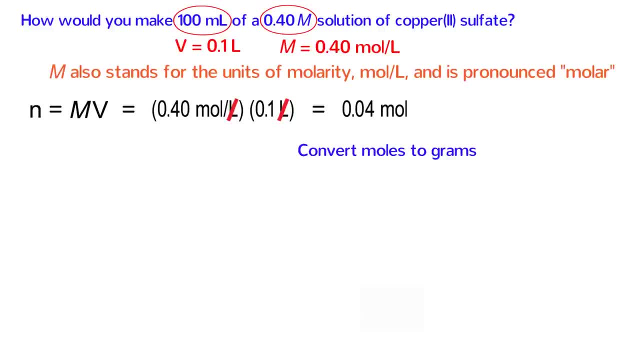 The easiest thing to do would be to look at the chemical label, which almost always has the molar mass written on it, But let's suppose we can't do that. The Roman numeral 2 means that the copper has a plus 2 charge and sulfate is SO4 2-. 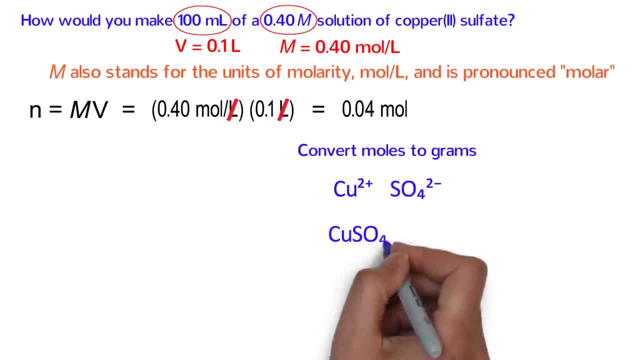 Because the charges are the same, the compound is simply CuSO4.. However, copper sulfate is almost always found as the pentahydrate, which means it has 5 water molecules that have co-crystallized with the copper sulfate. 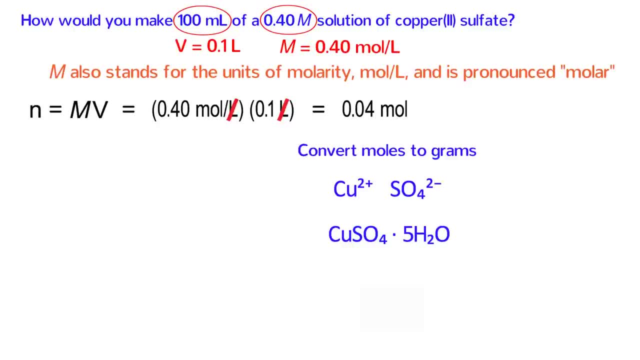 So we need to find the pentahydrate. These water molecules aren't really doing anything. they are basically just hitchhiking with the copper sulfate. However, these water molecules do affect the molar mass, which we will go ahead and calculate. 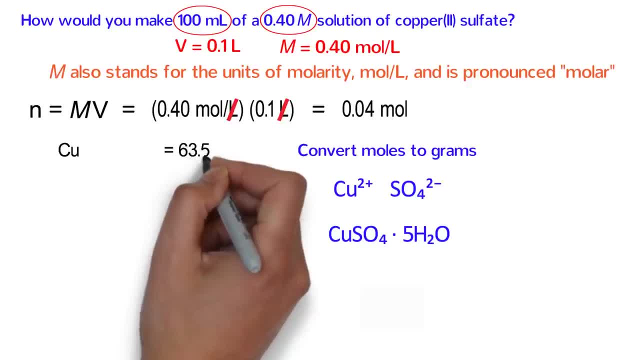 now The formula contains 1 copper with a molar mass of 63.55 grams per mole. 1 sulfur, which is 32.07 grams per mole, 9 oxygens. so we multiply 9 times 16, which equals 144 grams. 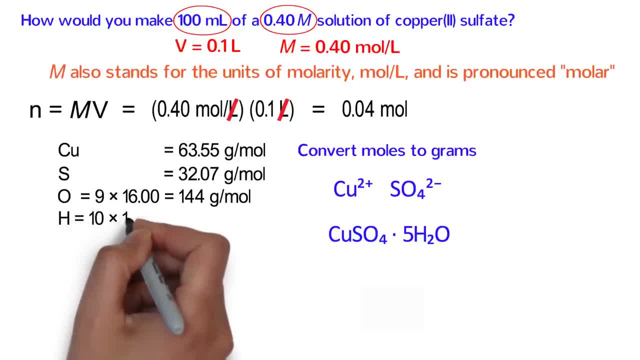 per mole and 10 hydrogens. So we multiply 10 times 1.008 to get 10.08 grams per mole. Add all these together to get the molar mass of 249.7 grams per mole. This is our conversion factor between moles and grams. 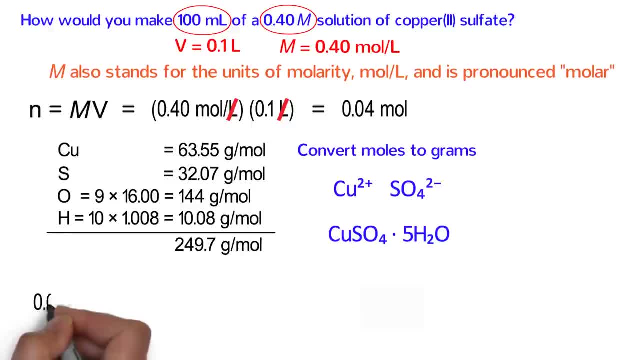 In order to calculate the mass of copper sulfate needed, we multiply 0.04 moles by a conversion factor fraction, Because we are starting with moles. 1 mole goes on the bottom Because we are solving for grams: 249.7 grams per mole. 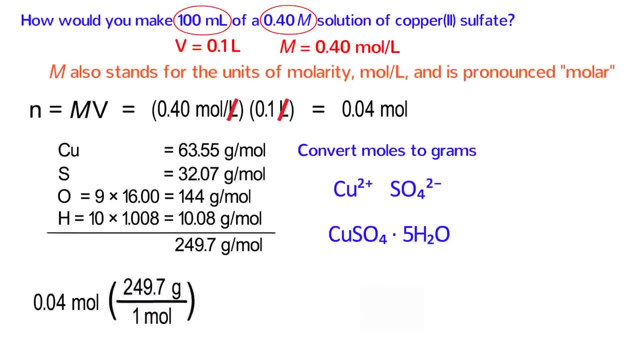 So we multiply 10 times 1.008 to get 10.08 grams per mole. 249.7 grams goes on the top. Moles on the top and bottom. cancel out Because the 1 is on the bottom. multiply 0.04 times 249.7 to get 9.988 grams. 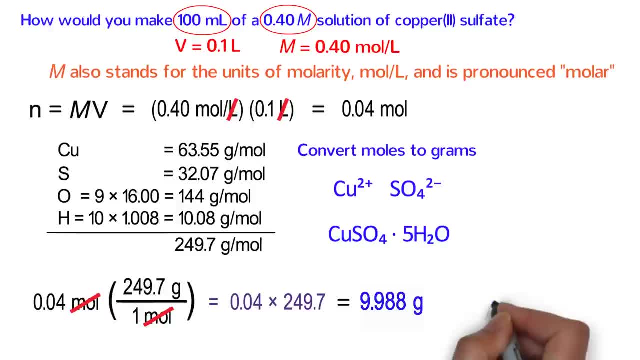 So how do you actually make this solution? First, get a 100 mL volumetric flask with a stopper. It should look something like this. Next, weigh out 9.988 grams of copper sulfate pentahydrate And carefully add all the copper sulfate.